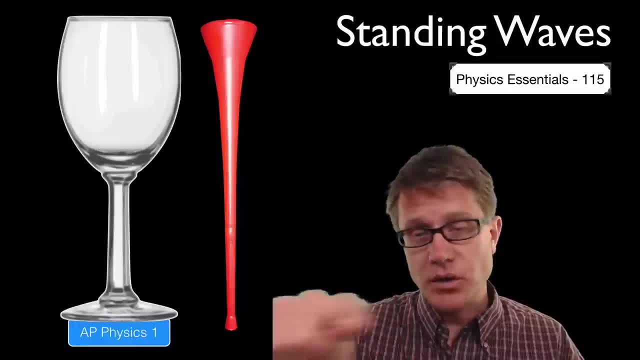 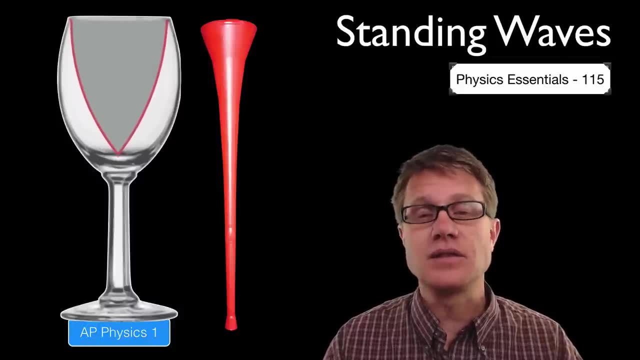 of the vuvuzela. Now, a wine glass works the same way. If you rub your finger with a little bit of water around the surface of it, what you can do is generate these standing waves inside the wine glass. What you are doing is vibrating the sides, And as you do that, 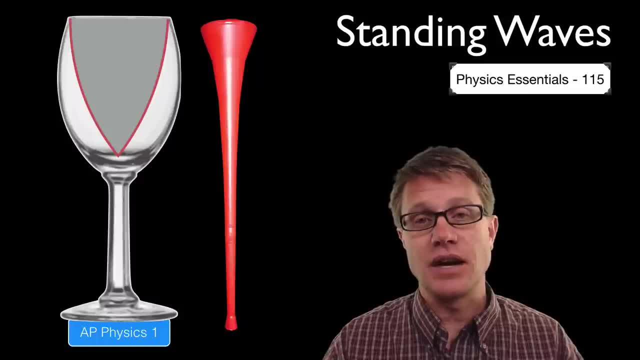 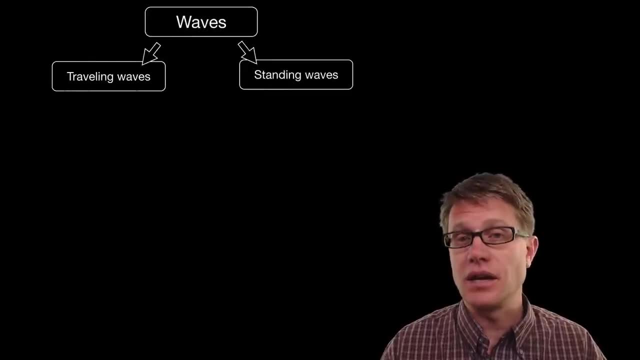 you are vibrating the air And since you have a standing wave inside there, it makes this pitch. Add water to it and you are going to have a slightly different pitch, And so waves can either be traveling or standing waves. Traveling waves will move from one place to another. 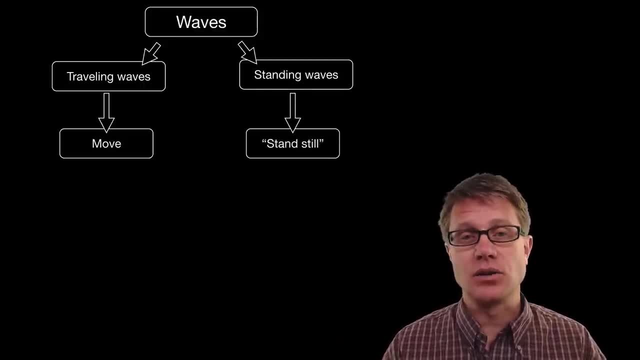 And standing waves will appear to stand still. Now, when you look at it, it is kind of an illusion. They are standing still, but the traveling waves are bouncing back and forth. In other words, they are being reflected off the boundaries and then there is interference to create these. 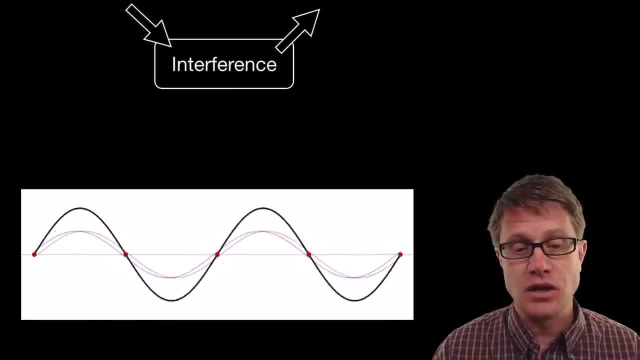 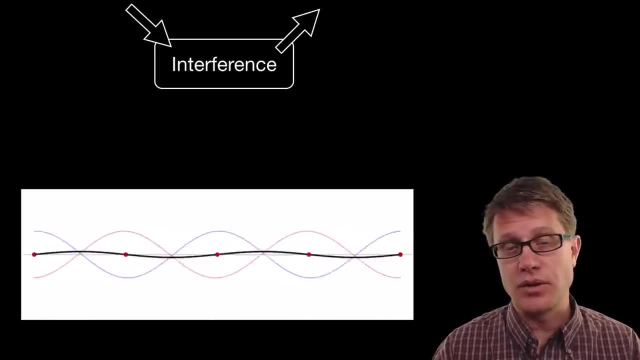 standing waves. And so, if we look at this animation, the dark wave is going to be the standing wave, But in the background you can see the blue and the red waves that are bouncing back and forth, and back and forth, And it is the summation. 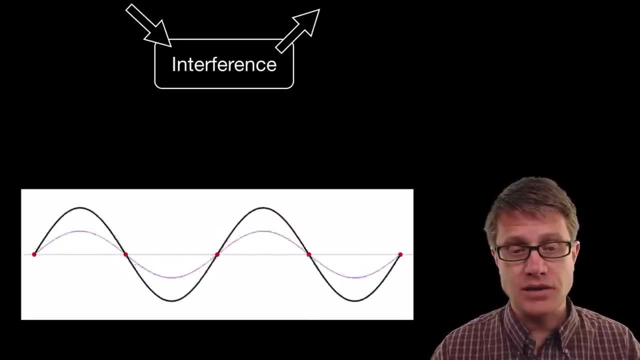 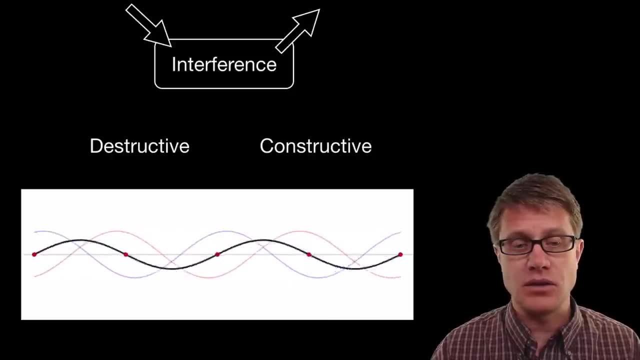 of them. that creates the standing wave. Now, if you notice that standing wave is going to have areas where it is not moving at all And that is due to destructive interference, where the waves are canceling each other out And we call those, in physics, nodes Areas- 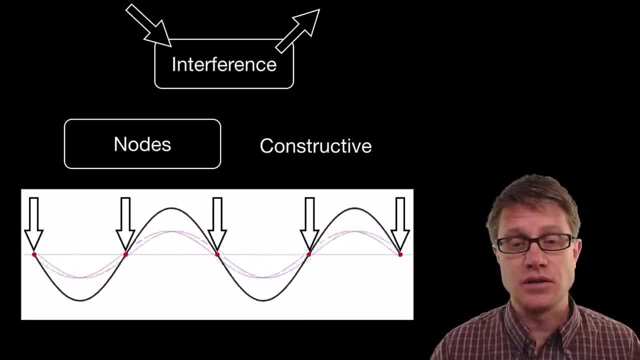 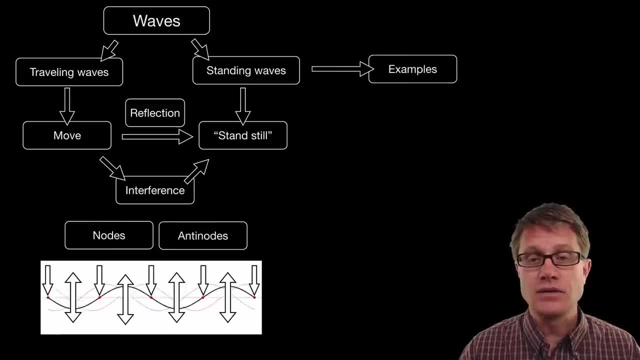 where it is not moving, And then we are going to have total constructive interference in certain areas And we call those antinodes. That is where it is moving the maximum amount back and forth, and back and forth, And so an example of this could be found in instruments. 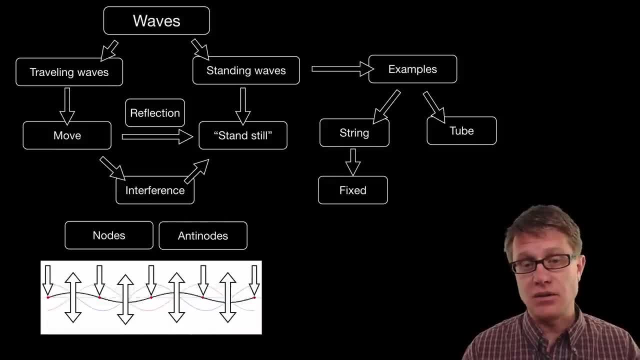 for example. So a string instrument is going to be fixed at either end, And this animation is a good example of that. It is fixed on either end And as the waves bounce back and forth and back and forth, you create these standing waves. If we shorten that, like on. 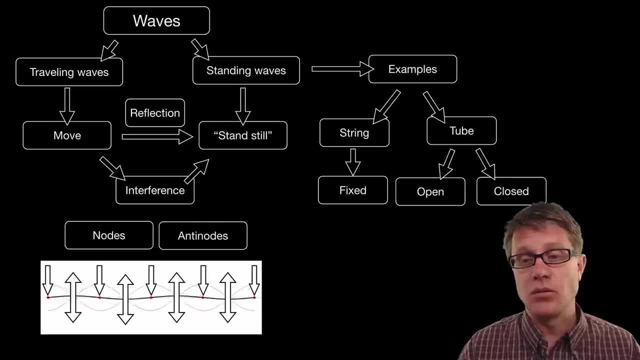 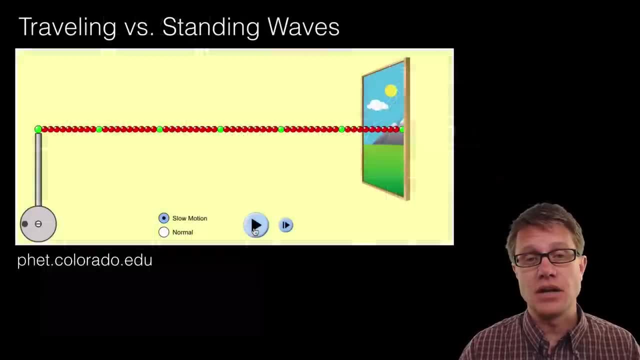 a guitar. then we can get different pitches. A tube is going to be the same way. A tube could be open on both ends, like a flute, or it could be closed on one end, like a vuvuzela, And that is going to create these standing waves as well. 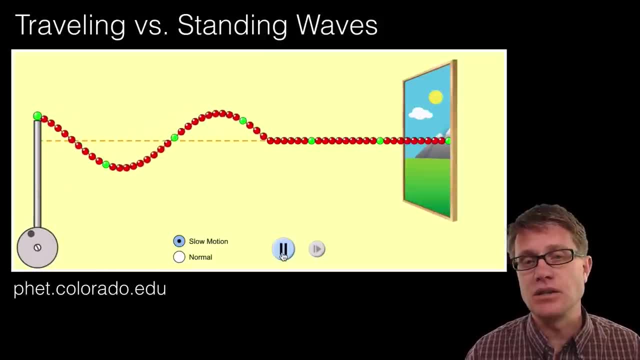 So let's start with traveling versus standing waves. And so this PHET simulation: I am generating some waves. Those waves- and this is just kind of theoretical- are moving out the door and then they have moved on forever. But if we add a boundary on the other side, in other 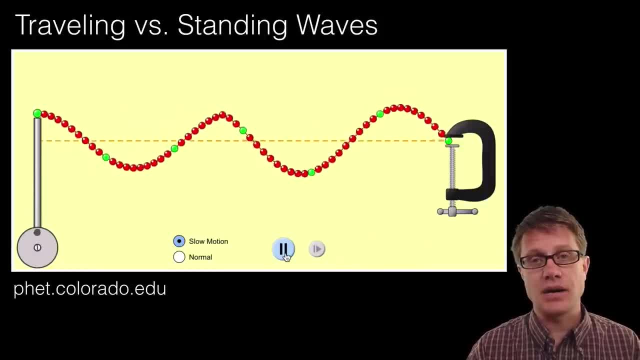 words if we add a fixed boundary. you can see now there is a reflection back. So those waves did not just keep going, They have bounced back, And now they are going to bounce back again. And as that wave goes back and forth, and back and forth, you can see that we are 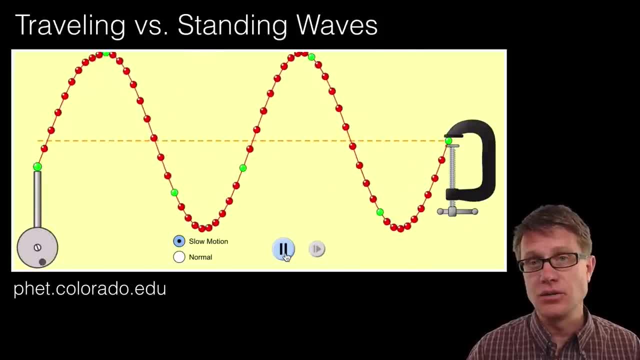 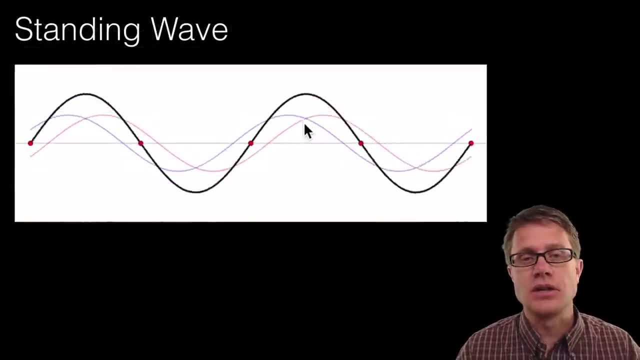 starting to generate these standing waves, And you can even see that we are starting to see those nodes and those antinodes, In other words, those areas where it is not moving and those areas where it is moving quite a bit. So this is an animation of standing waves. 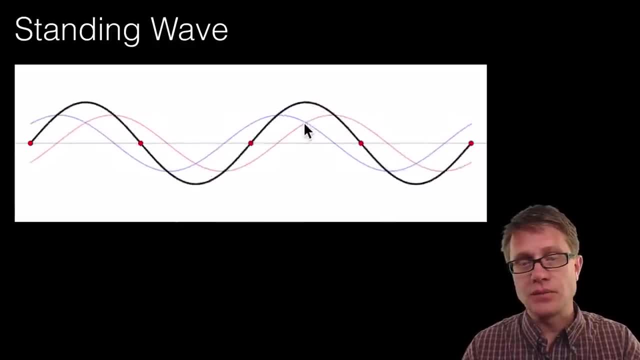 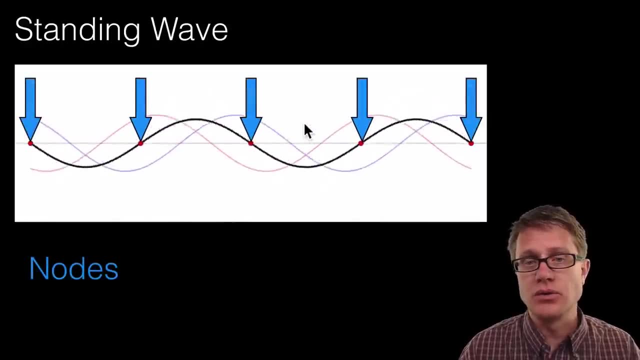 And so what we are doing is, as the blue wave moves to the right, it becomes the red wave, which moves back to the left, And it just keeps going and going and going. We are getting destructive interference That is causing these nodes where they cancel each other out. 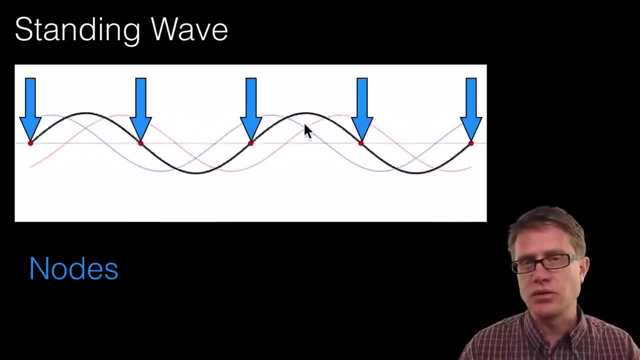 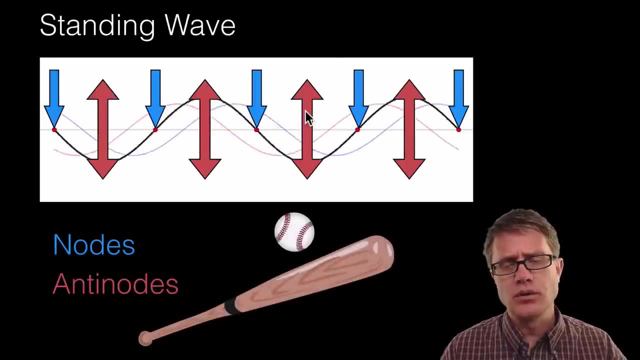 And then we have constructive interference and that is creating these antinodes, where those two waves add together to make a much bigger wave. Now an example of this: if you have ever played baseball before, when you hit the ball, sometimes you will hit it and the bat will kind of buzz in your hands. In other words, it vibrates. 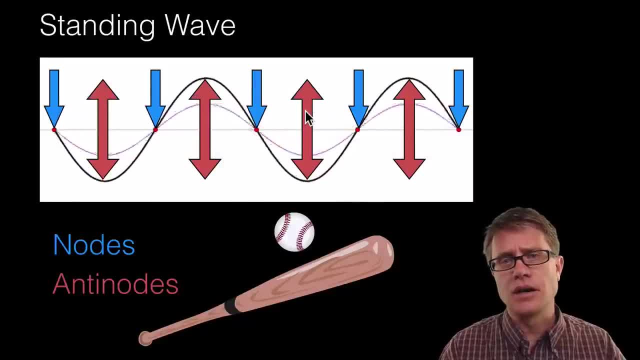 quite a bit, And the reason why is that you are hitting the ball on an antinode, an area where the waves going up and down the bat are actually constructively interfering to create a huge vibration there, And we refer to it as the sweet spot, the spot on a bat. 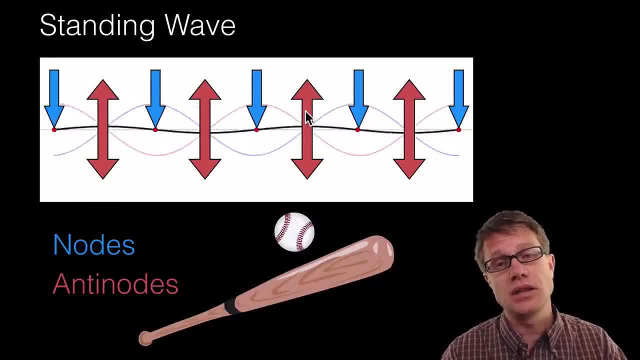 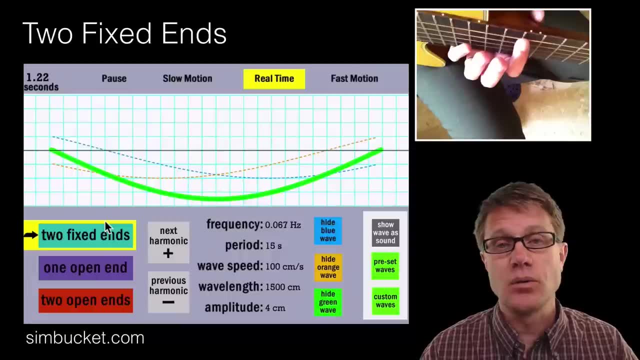 where the node is, where you do not have much vibration, that you hit the ball and you do not feel really any vibration at all. So that is what we are doing, And then we are going to look at this. So this is a sim bucket simulation. What we are doing is looking at standing waves. 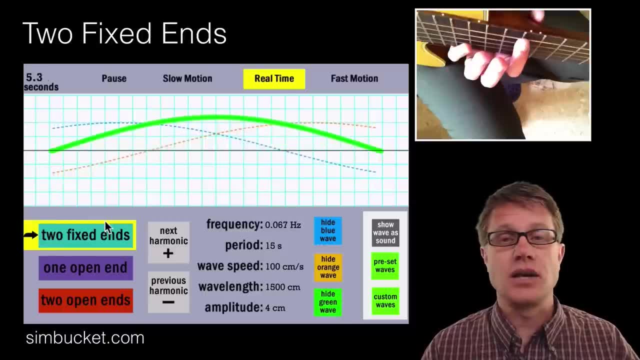 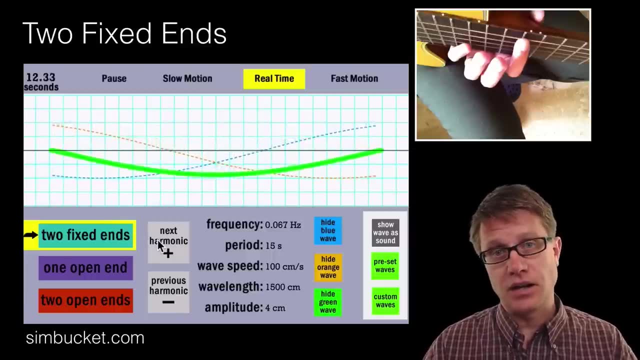 The first one we are going to look at is when you have two fixed ends. So an example of this could be a guitar, And so what you do is you have a string, you hold it on one side and then you pluck it and you are going to have vibration. So what do you get? Waves. 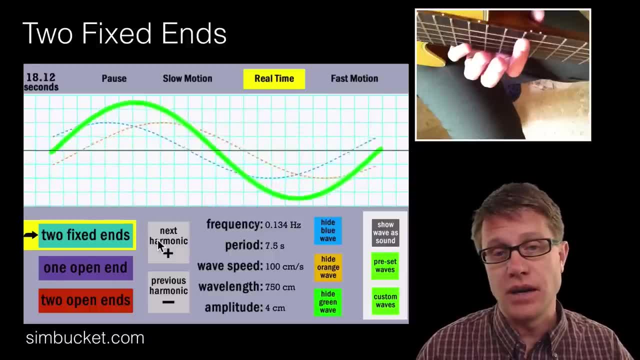 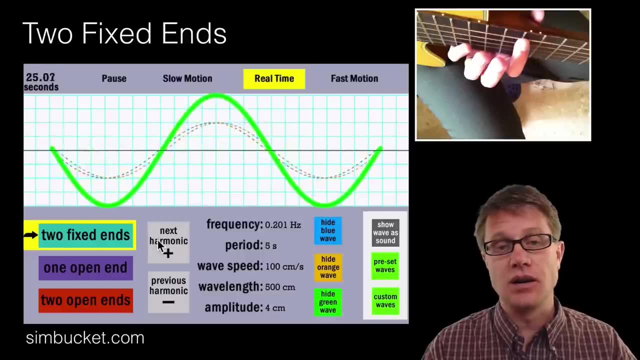 going back and forth, and back and forth. What is the standing wave then? The standing wave is going to be that green wave in this, in this simulation, It is that wave that is the addition of the other waves. What is interesting in a guitar is that you do not only have one. 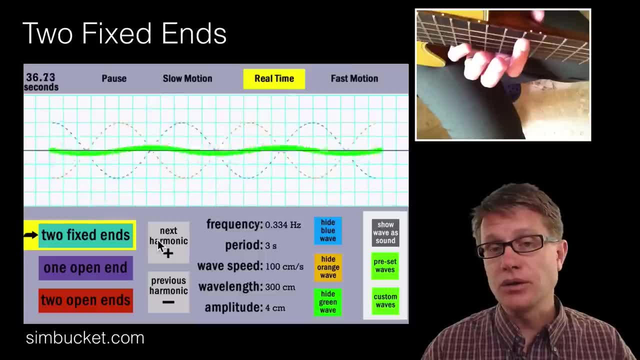 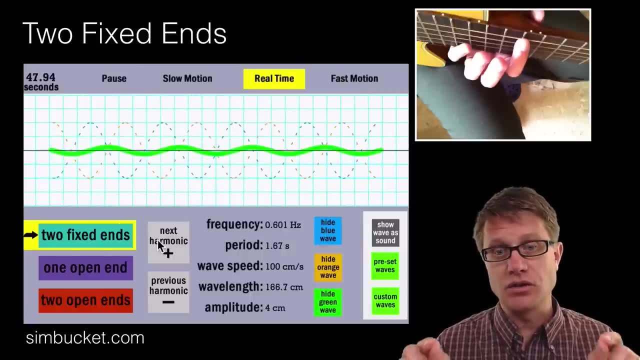 what we call harmonic or one standing wave, but you can have multiple standing waves. Now, in all these standing waves, what makes them the same is that we have a node on either side. In other words, there is no net movement on either side of that string, If we look. 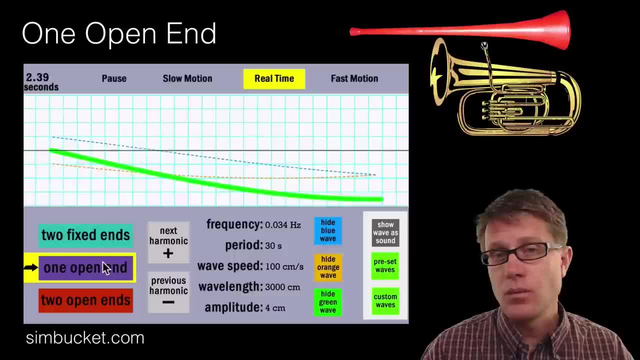 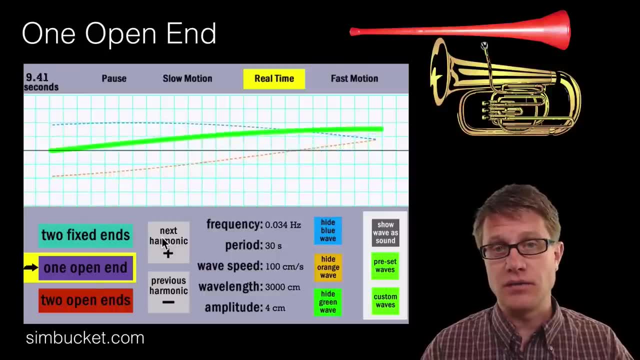 at an instrument like a tuba or a vuvuzela. what is the characteristic of that? Well, we are vibrating it, But you can see that on the left side we have a node. It is not vibrating But we have an antinode at the right side. So in each of these harmonics- the left side, 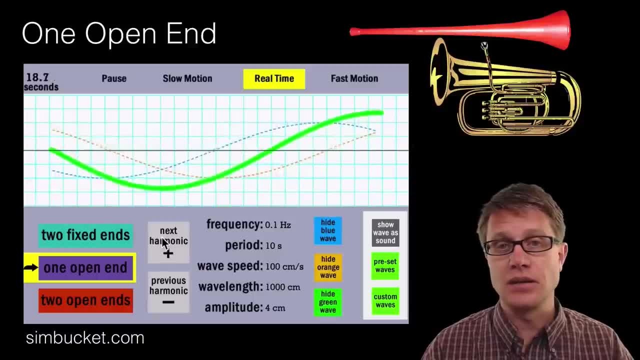 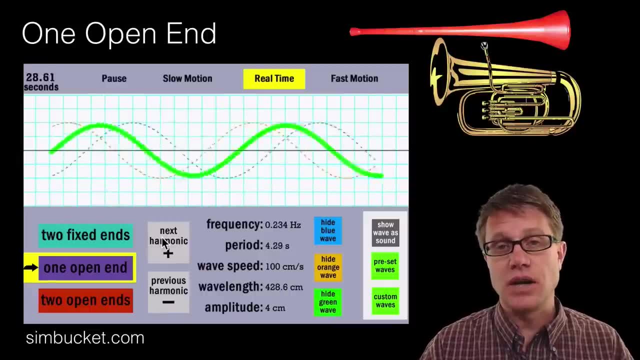 is going to be a node. It is not going to move at all, But the right side is going to be an antinode, And so we still have those traveling waves going back and forth, and back and forth. It is just that one of those ends is free to create an antinode, And then we 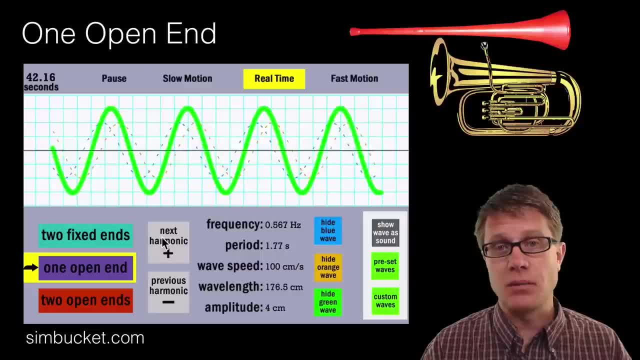 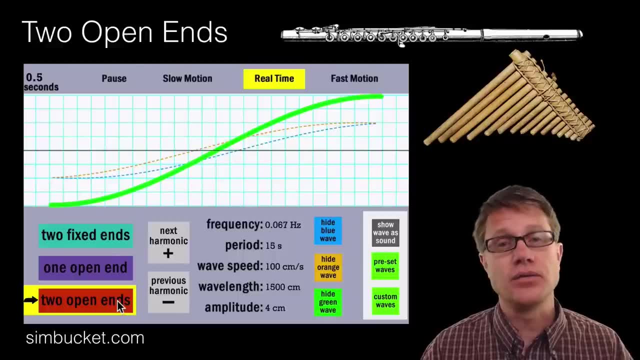 just have reflection off of that end. These are all the different harmonics. What keeps them all in common is the node: A node on the left, Antinode on the right. If we then look at something that has two open ends, like a flute- A flute, you do not blow in one end, You are blowing on the top. 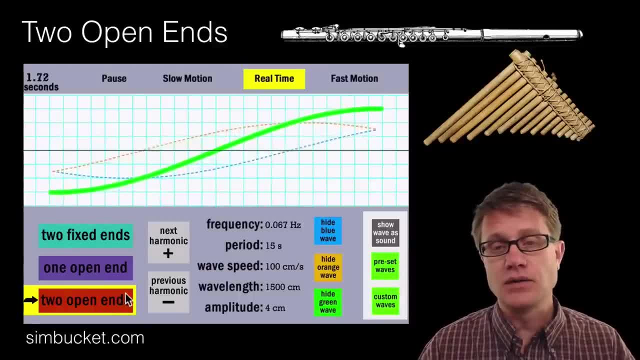 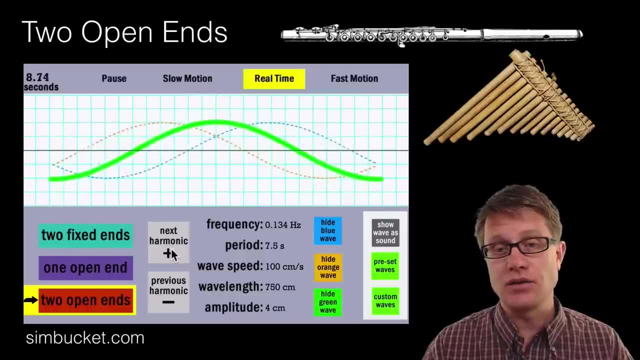 to create the vibration, Or a pan flute would be an example of that. And so what is going to create the standing wave here? Well, in this first harmonic we have the node in the middle, And then we have antinodes on either side. Now we have two nodes near the middle. 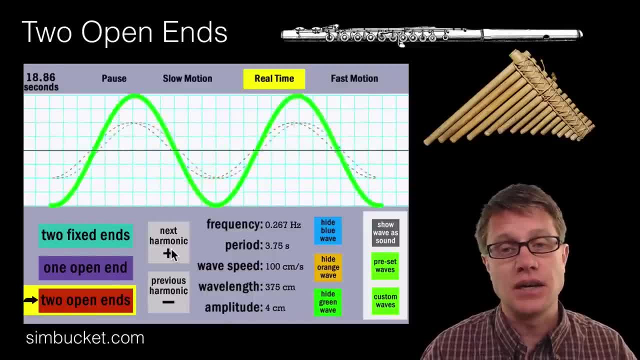 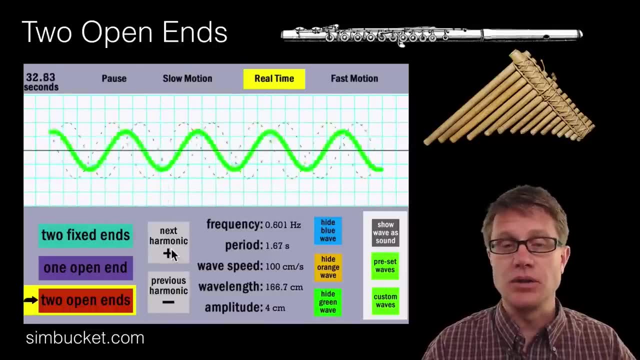 Antinodes on the side. So what is the characteristic of a standing wave in a chamber that has two open ends? It is always going to be an antinode on either side, But depending on the frequency we can get different pitches as we blow through Ruben's. 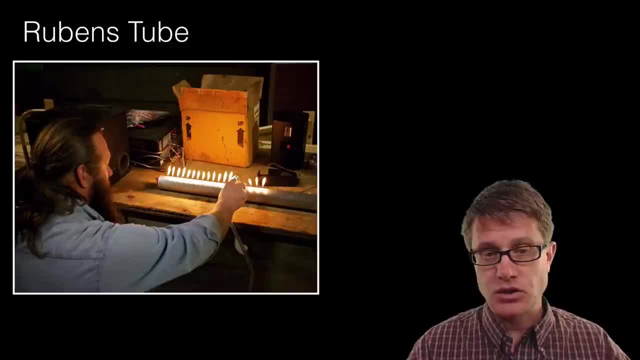 tube is a really cool example of that. In a Ruben's tube, what you do is you fill up a chamber with gas- A gas that is flammable- And so this guy is lighting the chamber. So we are having flames coming out of the top, But on a Ruben's tube you put a speaker on. 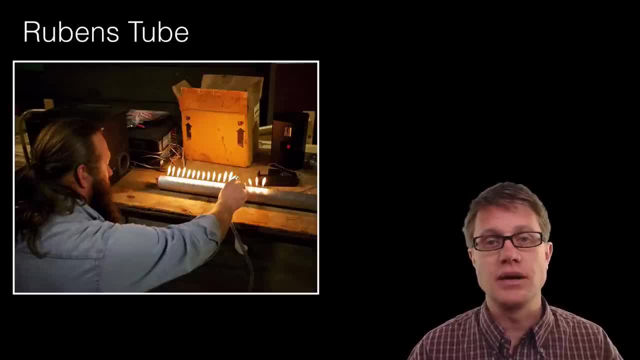 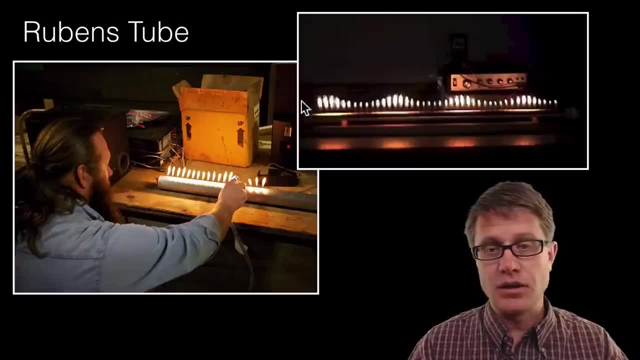 the side And what that speaker does is create these longitudinal waves. Those longitudinal waves as they move through will create areas where there is a lot of compression And an antinode. is where there is a lot of compression or antinodes, Then the gas really cannot make. 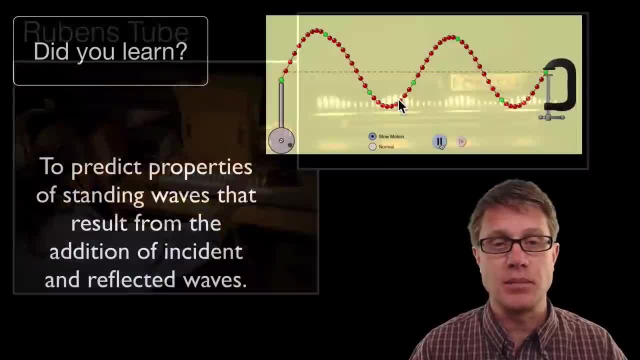 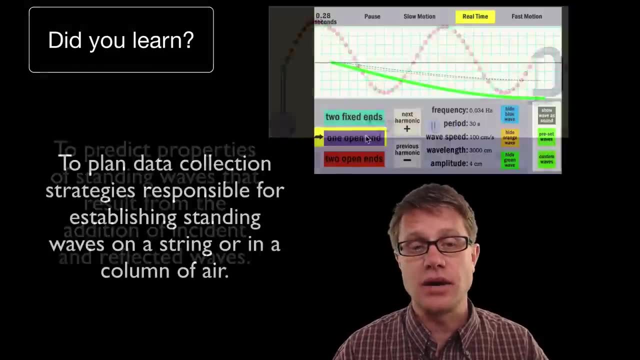 its way out, And so it will be really low there. But at the nodes it will actually come out quite a bit. And so did you learn to predict the properties of standing waves. They result from reflection of these traveling waves. Could you collect data? Again, I used a sim. 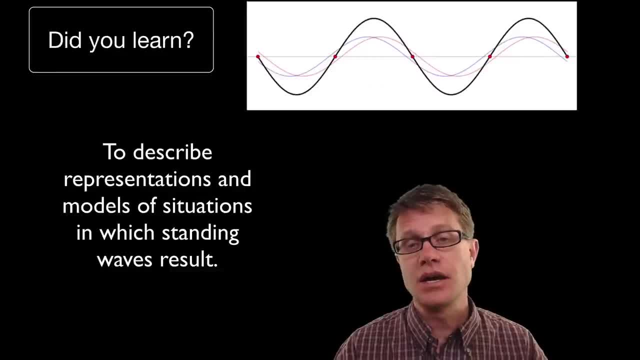 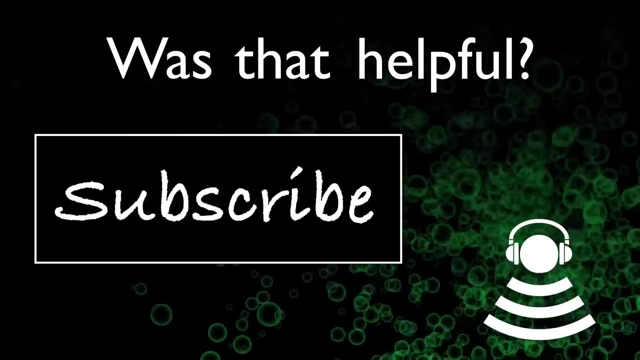 bucket simulation to do that? And then, finally, could you describe examples of when this occurs? standing waves. Musical instruments are good, Baseball bats are great, And I hope that was helpful. Thank you very much.